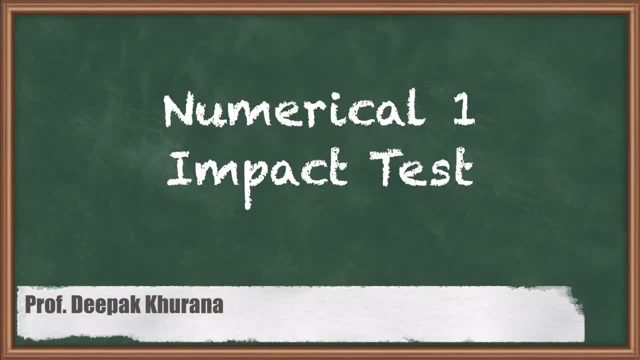 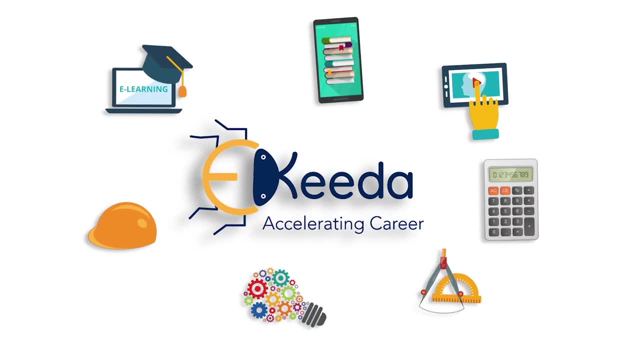 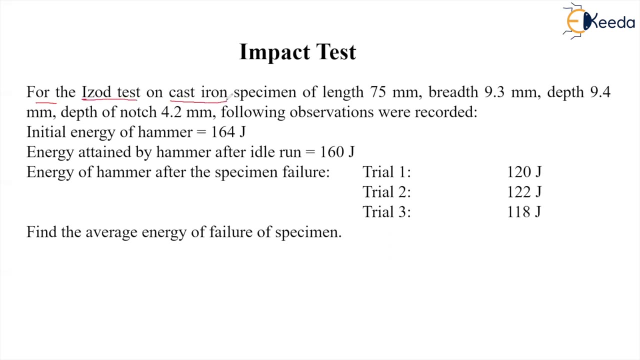 Hello students, in this session let us have one example of impact test For IZOD. IZOD impact test is there. For IZOD test on the cast iron specimen is there. Length of the specimen is 75 mm. breadth is 9.3 mm. depth is 9.4 mm. 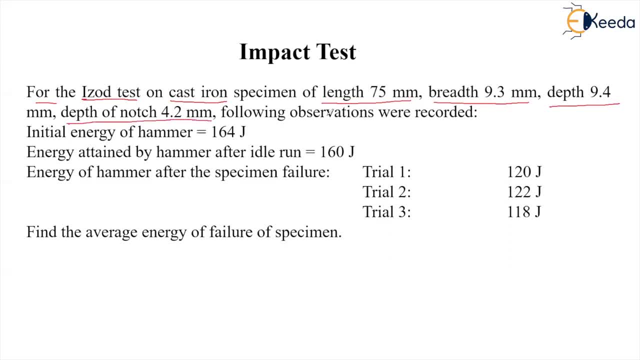 And depth of the notch is also given 4.2 mm. Following observations were recorded. What are the observations? That initial energy of the hammer, when the hammer is placed at its original position, that is 164 joule. Basically, this is obtained from the height using the formula MGH. 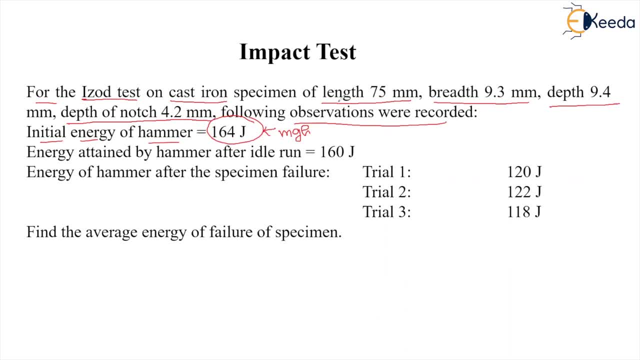 H is the height of the hammer above the datum. So using MGH we have given the direct value of the energy. 164 joule is the initial energy of the hammer When the idle run is done. idle run is done, it means that. 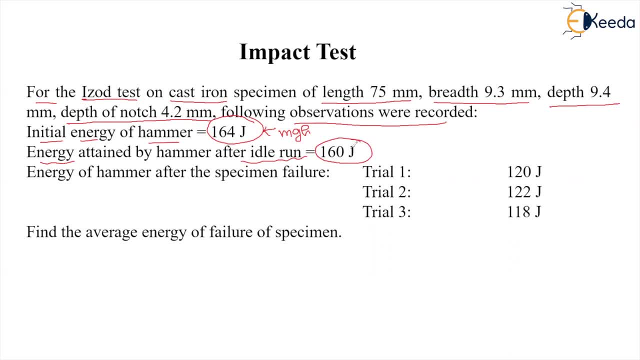 it is getting 160 joule of energy right. It is not getting 164 joule because there is some friction in the air and some energy is lost in the air, right. So we have to consider also the friction losses in this case. So 160 joule of 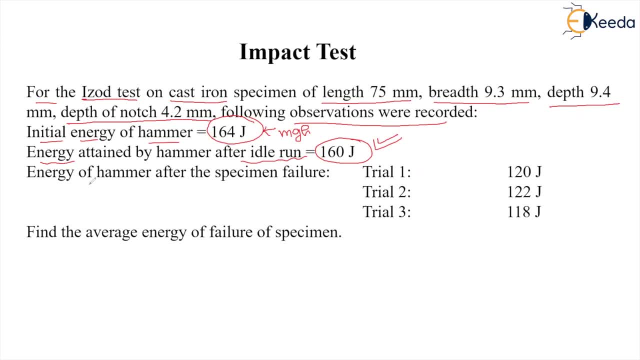 the energy is there when this is idle run And energy of the hammer after specimen, failure right. So in failure some energy is lost and after the failure takes place, the energy obtained is 120 joule in first trial. 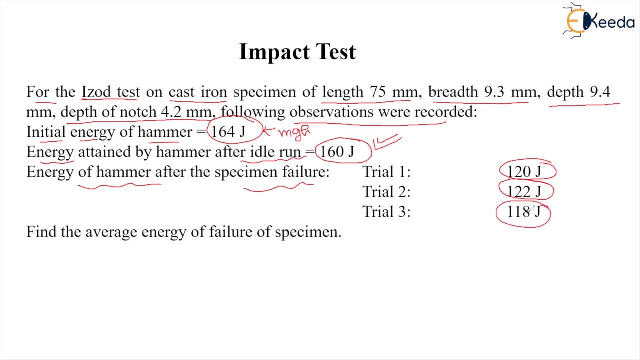 270 joule in second trial and 1180 joule in third trial. We have to find the average energy of the failure of the specimen. how much energy is consumed in the failure of that specimen? So let us solve this question. 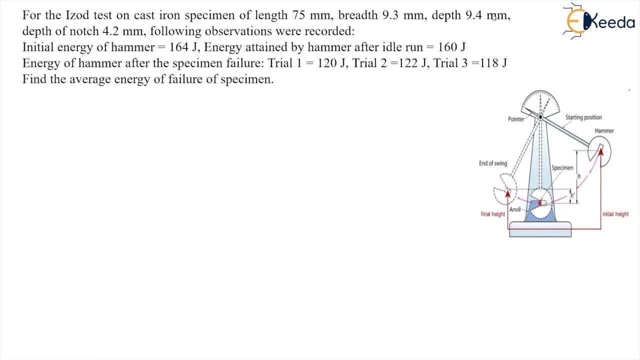 In this question we are given with specimen. the dimensions of the specimen are given to us, which is not important for us. it is given that initial energy of the hammer is 164 joule, So it means that the hammer has an initial energy. the height is there, they have. 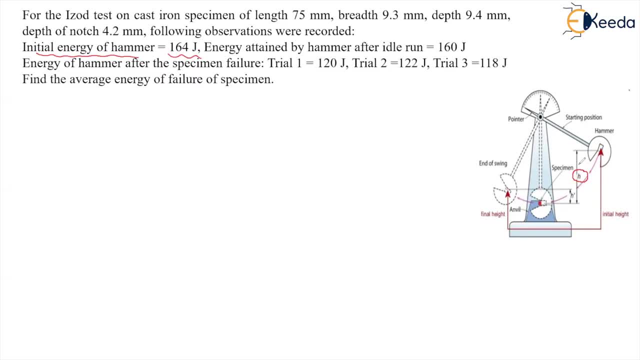 directly obtained, given us the energy in terms of joules rather than giving the height. So in some cases height also may be given and you have to find the initial energy using the formula mgh, right. So initial energy is given to us, that is, the 164 joule. in this case it is given to us. 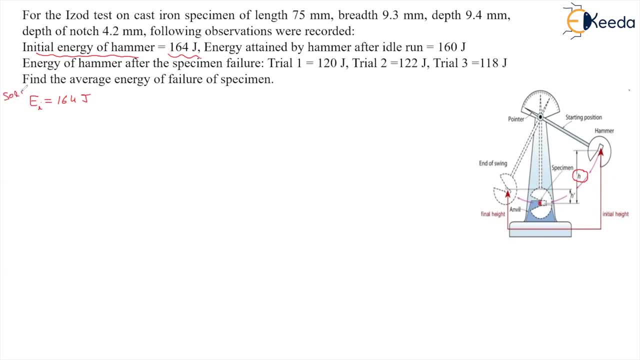 right. Next, this is also given that the idle run. in idle run, the energy obtained is 160 joule means when we are doing idle run, we have left this hammer freely, without breaking the specimen. it will move to another side. 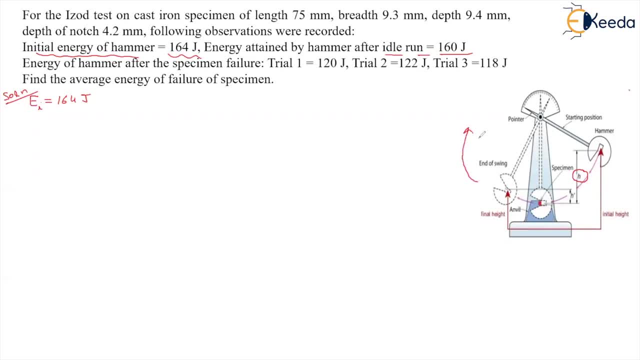 It will move to another side and it will receive a certain height, but the height received is less than the actual initial height of the than that hammer, because there is some friction also right, So we can write that the in idle run, idle run, the energy, energy for idle run. 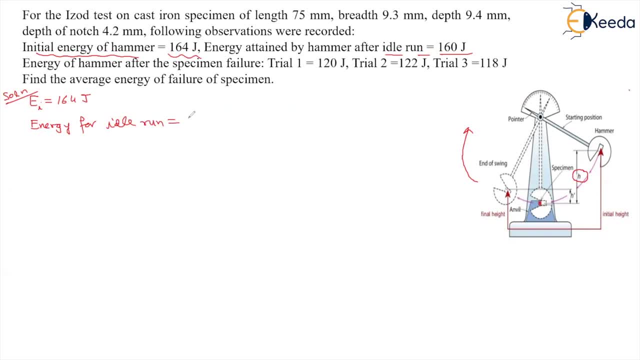 that is 160 joule, 160 joules right. So it means the energy lost in fiction is energy lost in friction, in air friction. So some energy is lost in air friction. So energy lost in air friction is that is equal to: 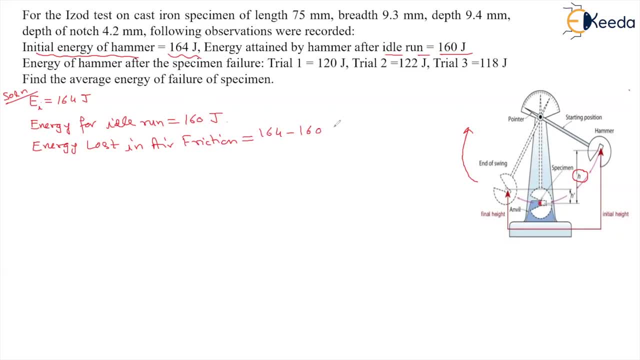 164 minus 160 joules, So this will be equal to 4 joules. So 4 joules of energy is lost in air friction. is it okay now? but this energy lost is is to is both sides means when the swing is the our pendulum. 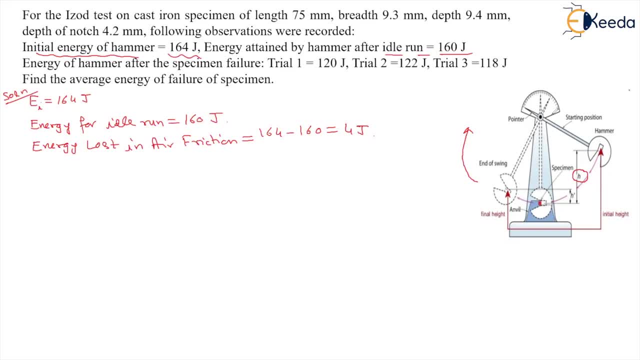 is on right side as well as on the left side, because from one side to another side it will pass from the two sides right. so average energy loss: we have to find out. so average energy loss in friction, average energy lost in friction, basically air friction here. so that will be. 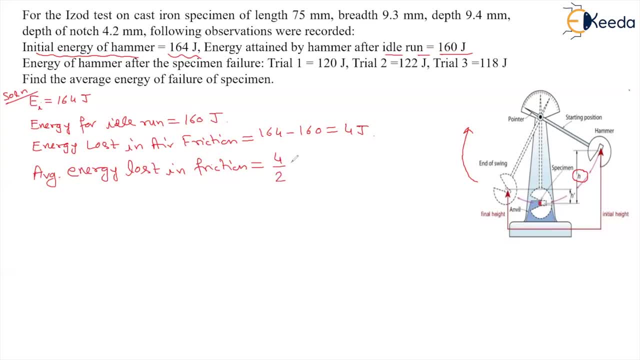 equal to total energy divided by there are two passes, are there? so this will be two joules. so two joule of energy is lost on right side, and two joule of energy is lost on left side. now then, the trial is done with the specimen in. 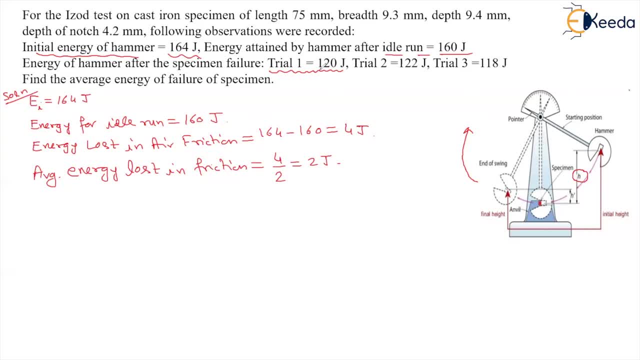 trial one: the energy obtained after failure. it is in the energy of the hammer after the specimen. failure is given as 120 joule. it means that some energy is lost in friction and some energy is lost in breaking the material and and finally we have got the 120 joule of energy right. 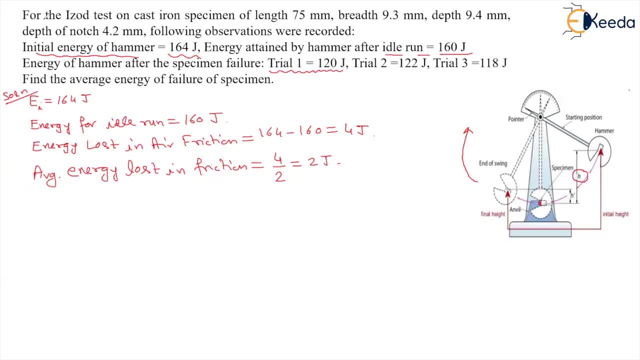 so in trial one. so in trial one, trial one. what is happening is. what is happening is, and the energy of the specimen is given to us, energy of hammer, basically right, energy of hammer after failure. after failure of the specimen means after failure of the specimen, failure of specimen. 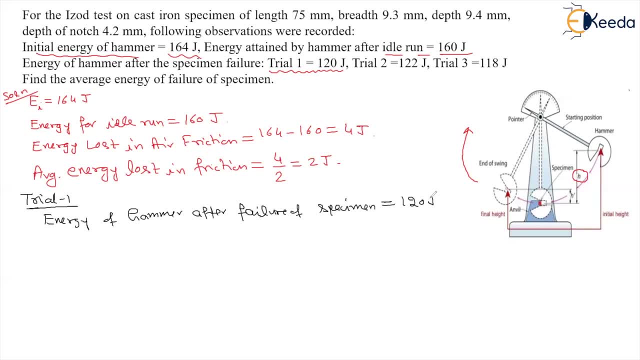 this is given to us. that is 122, right. it means energy lost, so total energy lost. i'm writing total energy load and this total energy loss will be having two components. total energy lost is out of this: 164 joule, 164 joule. total energy lost is: that is minus 120, 164 minus. 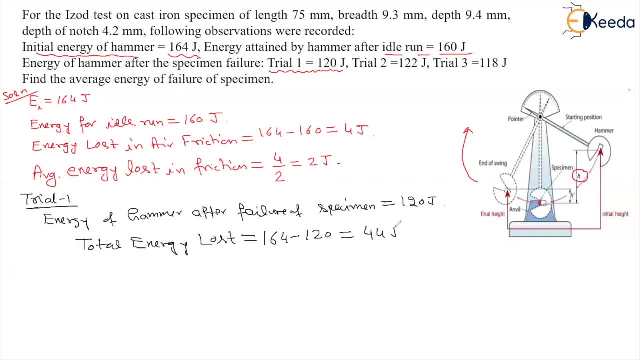 one quantity, so this will come out to be 44 joules. so this is the total lost energy: 44 joule. and this 44 joule composed of two components: the energy lost in breaking the specimen and energy lost in friction. so so this total energy lost, total energy lost having two components. one is the 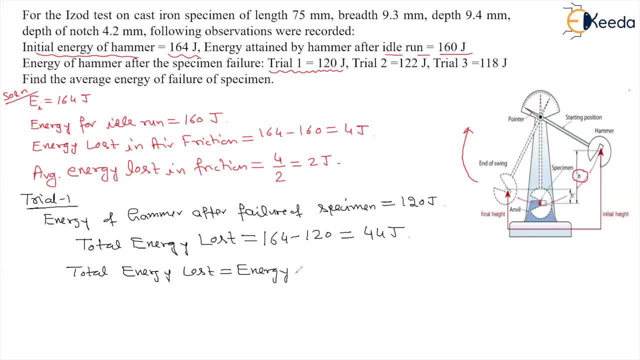 energy lost in breaking the component, energy lost in its need breaking- and you can take the load out of this ЭΔ- and energy lost in friction watts as took, and energy loss in air friction. we already know that it is a result of loss in friction loss. 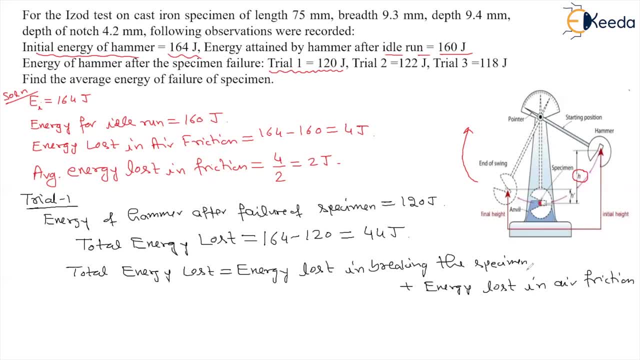 you play water, Namely this loss, EI. your once EI. you always liked Na which willравja, but we have to dedicate EI to a dysmethvem. Fli often is not so EI, but when energy is lost in it, then we will use friction, we will useมาsyan. it is general energy, but the signal provides moisture is high. so then it will come into the amount of energy loss and energy-how. im moving air friction right if energy loss in it means so that the energy loss in the end- we know that air friction is additional, that energy loss is outside this. if you are without a constant energy loss, the energy loss and there is noשre~. 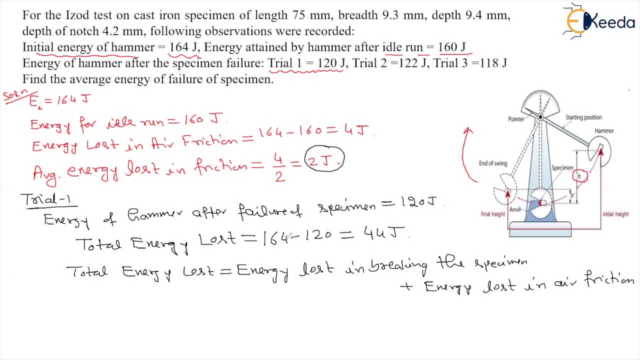 2 joules right. so approximately we can use the 2 joules of frequency, right. so then, what is the energy lost in breaking the specimen? so energy lost in breaking the specimen. so what is the energy lost in breaking the specimen? so energy lost in breaking of specimen. 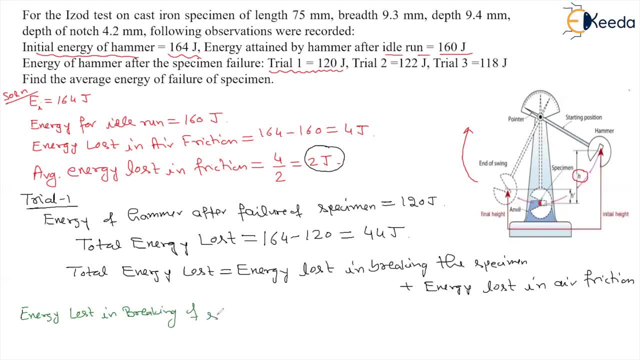 taking out specimen. so that will be equal to total energy. total energy. after the total energy, some energy is lost in air friction minus friction loss. friction loss right. so total energy is 44 joule in this case, minus 2 joule of energy. average energy lost in friction: 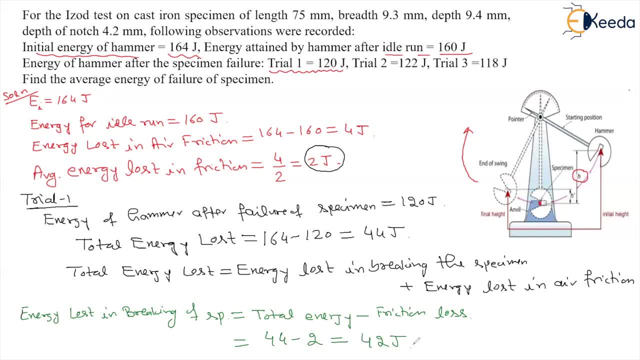 so that will be equal to 30 joules. so if we try to sprinkle 300 joules of energy into 42 joules, So one answer of this question in trial run is that the energy lost in breaking the specimen is 42 joules. Similarly, in trial two, some energy lost will be there. Similarly. 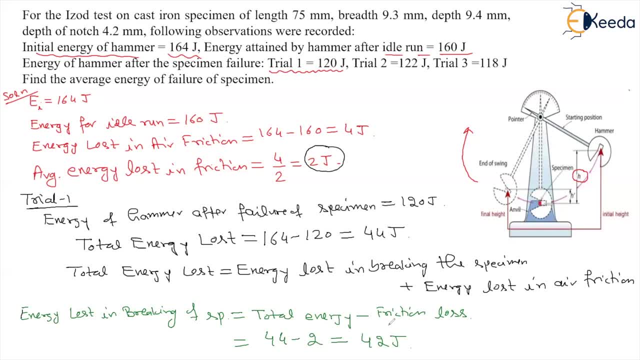 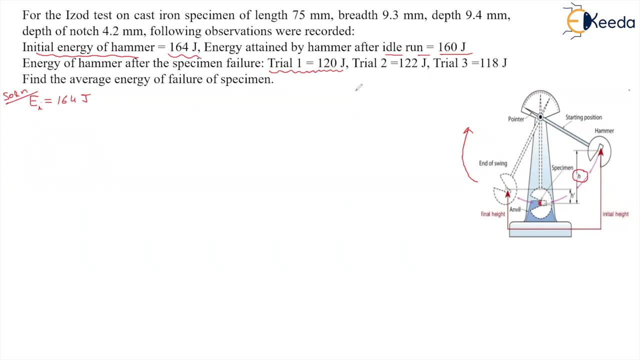 in trial third, some energy lost will be there in breaking the specimen. Three trials are there. Now we will do the trial two, what is happening in trial two. So this is the trial number two. Similarly we will do. the energy lost in trial two is 122 joules, So 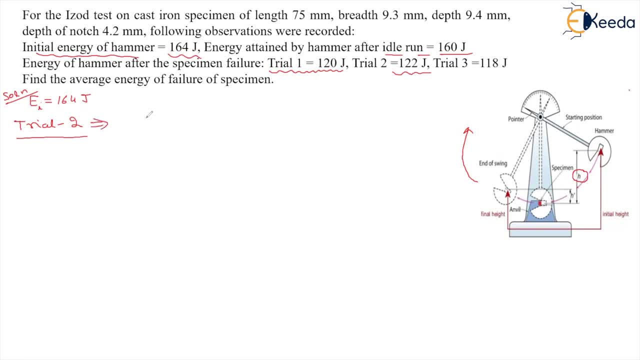 energy of the specimen is 122 joules. So energy of the hammer- hammer After failure, after failure of the specimen- is 122 joules. So energy lost, total energy lost: how much is the total energy lost Which is having two components? that is equal to. 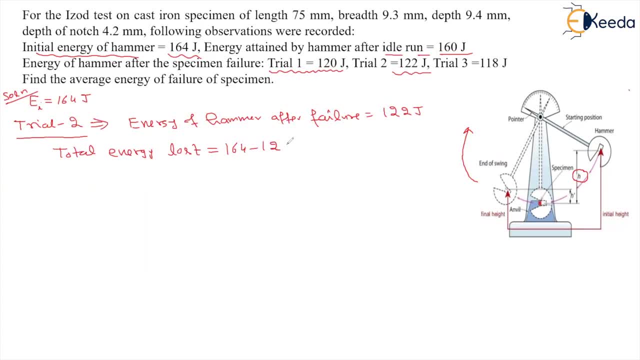 that is 164 minus 122.. So that will come out to be 42 joules. This much energy is there is lost in total. Then what is the energy lost in failure? Energy lost in failure of specimen Specimen that will be equal to this energy: total energy minus some energy loss. 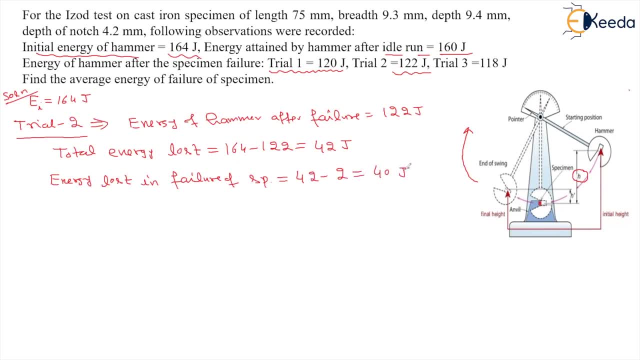 in friction, air friction, So that will be 40 joules. So 40 joules energy is obtained in this case right In trial one. how much was the energy? That was 42 joules. That was 42 joules. 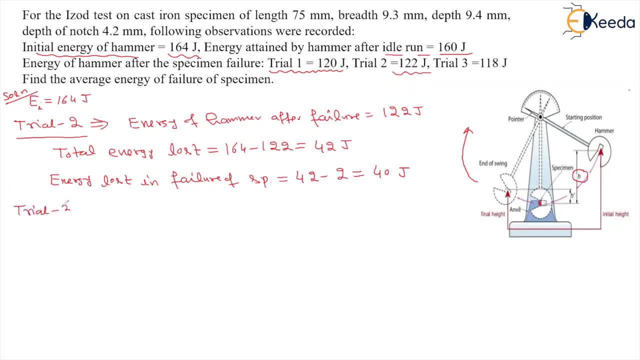 Now in trial 3, what is happening in trial 3, so energy of the hammer is given to us, that is 118,. so energy of hammer after failure is obtained to be that is 118 mu. this is the energy of the hammer after the failure takes place, that is 118 mu. failure of the 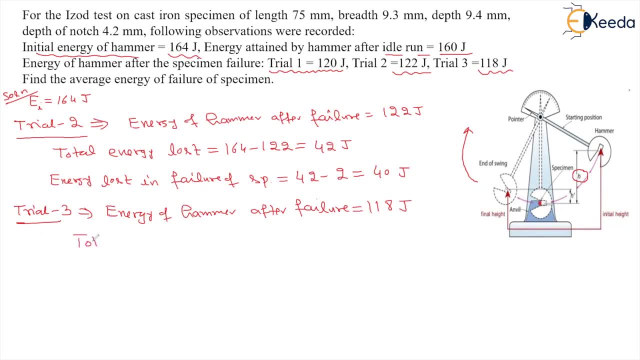 specimen 118 mu, then total energy lost. total energy lost, so that will be equal to: out of 164, 118 mu is lost, so that will come out to be 46 mu, 46 mu and this 46 mu composed. 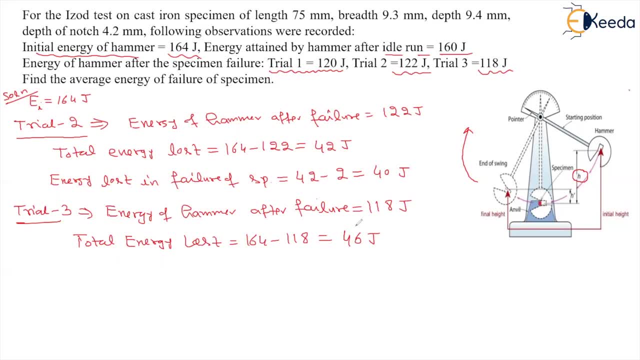 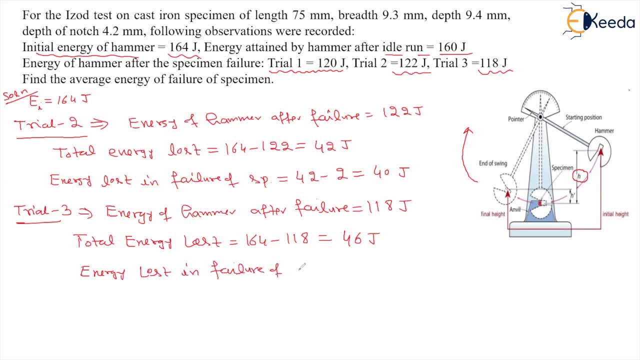 failure of specimen. that will be equal to. that is 46 minus the average energy of the friction friction loss. that is, for 2 mu that is come out to be 44 mu. And in trial 1, we have already done, trial 1, we have already done- 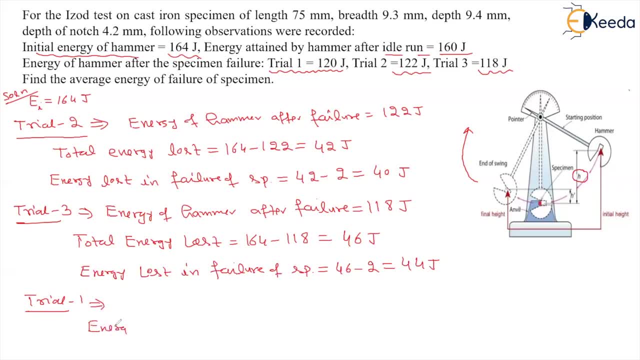 And in trial 1, the energy lost in energy lost in failure of specimen was was come out to be 42 joules. So now 3 experiments are done, 3 runs were there and in first run the 42 joule energy. 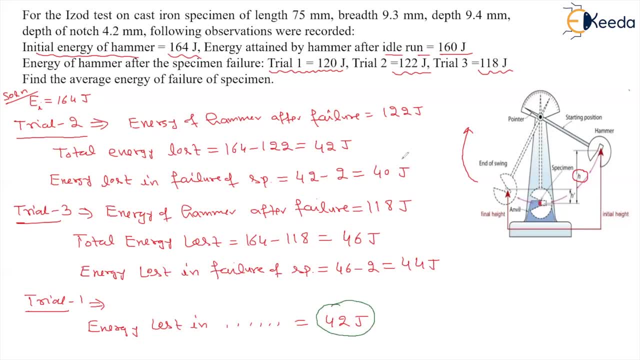 was lost in the failure of the specimen. in the second run, 40 joule of energy was lost in the failure of the specimen, and in third trial. In third trial, 44 joules of energy was lost in the failure of the specimen.